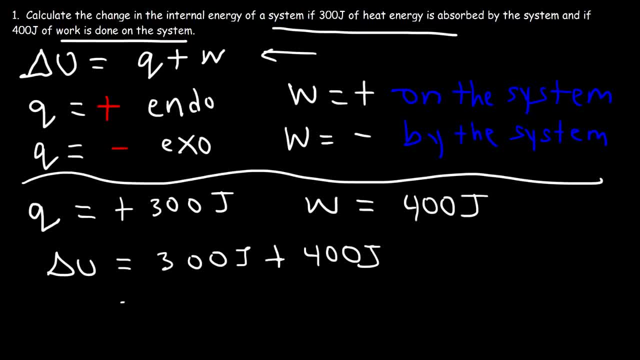 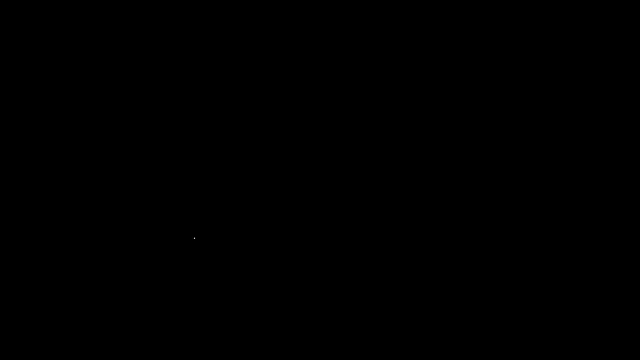 So both of these events work to increase the internal energy of the system. So the change in the internal energy is 700.. So if you want to draw a picture, let's say inside the box represents the system and everything outside of that is the. 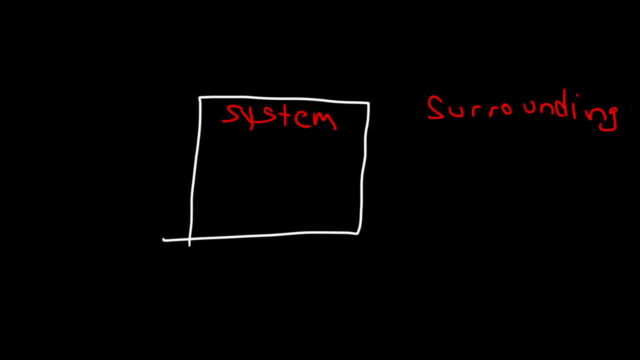 surroundings. So the system absorbs 300 joules of energy. So the system gains 300, which means the surroundings loses 300 joules. So this process is endothermic for the system. So the system gains 300, which means the surroundings loses 300 joules. 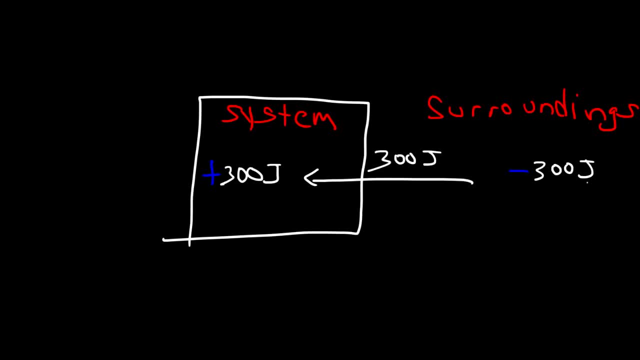 We put 400 joules of heat on a system but exothermic for the surroundings. Now work is done on a system. 400 joules of work is done on a system, So the system gains 400 joules of energy. 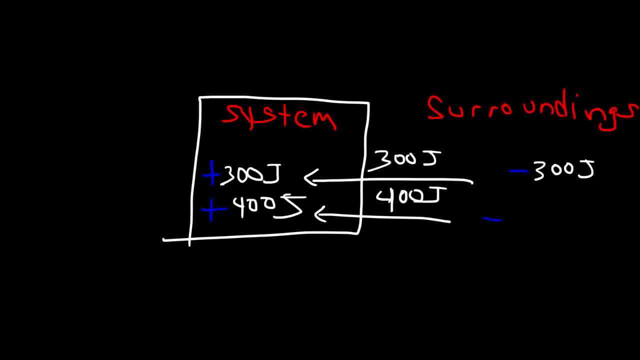 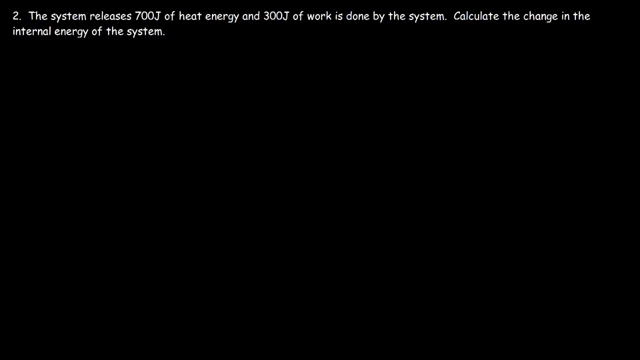 With the surroundings, loses 400 joules of energy through work. So we could say work is done on a system, but work is done by the surroundings. Let's try this one. The system releases 700 joules of heat energy and 300 joules of work is done by the system. 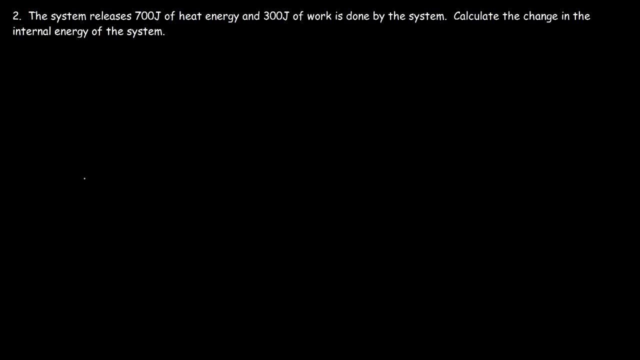 Calculate the change in the internal energy of the system. So let's start with a picture first. So this is going to be the system, and outside of that we have the surroundings. So the system releases 700 joules of heat energy. So 700 joules of heat energy transfers out of the system. 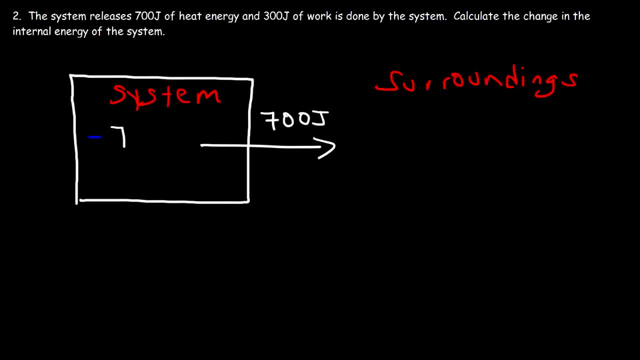 So this is going to be negative 700 for the system because it lost that energy but the surroundings gain 700 joules of heat energy. Now 300 joules of work is done by the system. If the system is doing work. 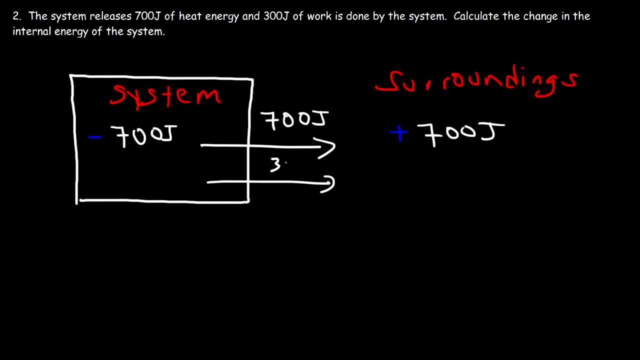 it's a condition that the system is doing work, So it's expending energy to do that. So the system is going to lose another 300 joules of energy, but the surroundings will gain that 300 joules of energy. So the surroundings gain a total of 1,000 joules. 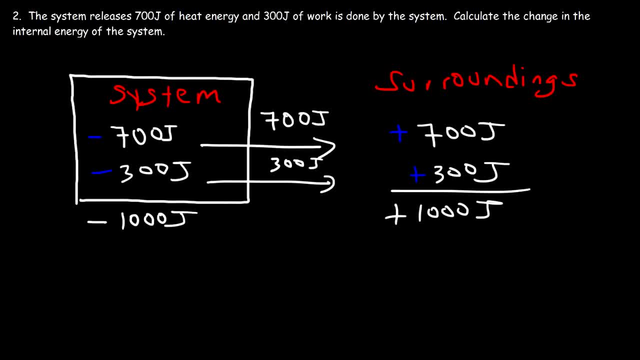 but the system loses a total of 1,000 joules, And so we have the first law of thermodynamics. Thermodynamics, energy is neither created nor destroyed. It's simply transferred from one place to another. So delta U- I forgot the U. 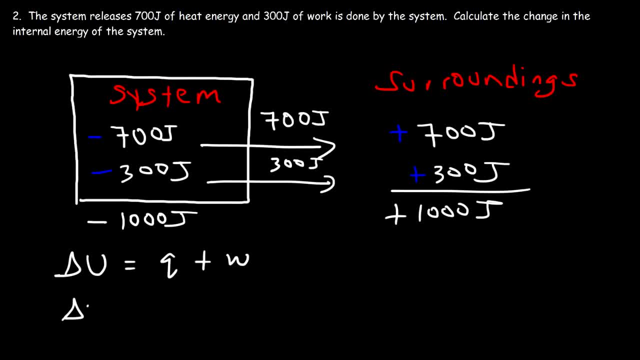 which is Q plus W, it's going to be negative 700 plus negative 300.. So the change in the internal energy of the system is negative 1,000.. So if the system loses 1,000 joules of energy, the surroundings gain 1,000 joules of energy. 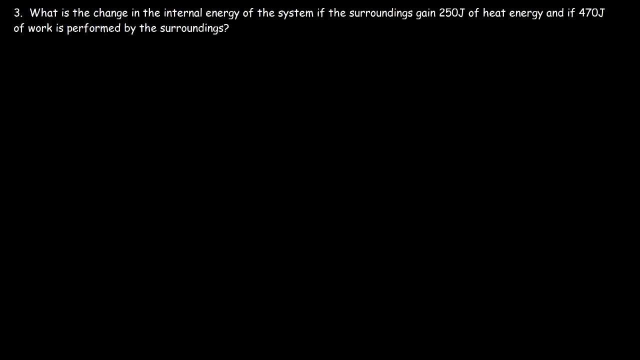 But this is the answer to the problem Number three: what is the change in the internal energy of the system if the surroundings gain 250 joules of heat energy and if 470 joules of work is performed by the surroundings? So you need to visualize the transfer of energy. 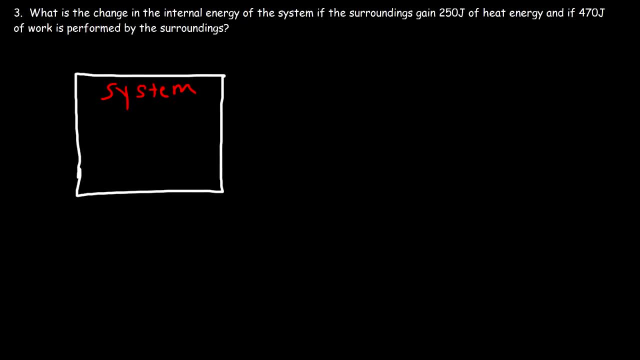 So if the surroundings gain 250 joules of energy, is that heat energy flowing into the system or into the surroundings? That energy is flowing into the surroundings, If it flows, if the surroundings gain that energy. So therefore we could say Q with respect to the system. 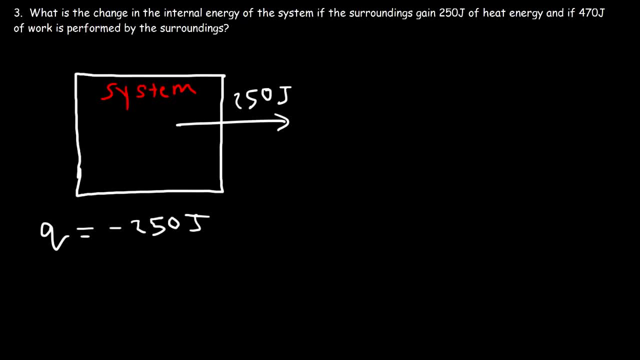 is negative 250 joules because heat energy is coming out of the system and going into the surroundings. Now, 470 joules of energy is flowing into the system. Now, 470 joules of work is performed by the surroundings, Whenever something performs work. 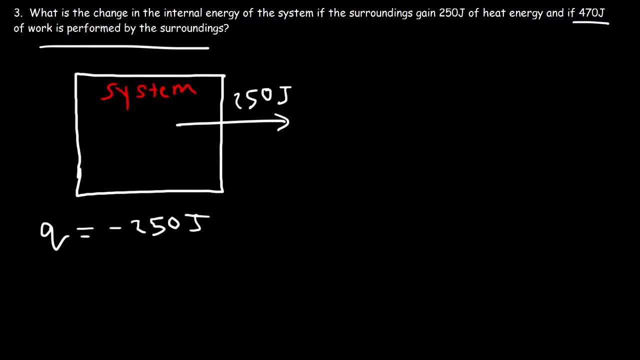 it loses energy to do so. For example, if you perform the work required to lift weights, you have to burn energy to do it. So if the system is doing work, the system is losing energy. So energy is transferring. I mean if the surroundings is doing work. 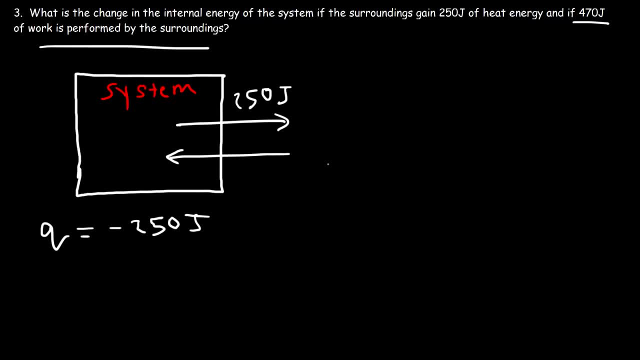 the surroundings loses energy, which means energy is transferred from the surroundings to the system. So we got 470 joules of work leaving the surroundings going to the system. So W is positive 470.. So delta U, which is Q plus W. 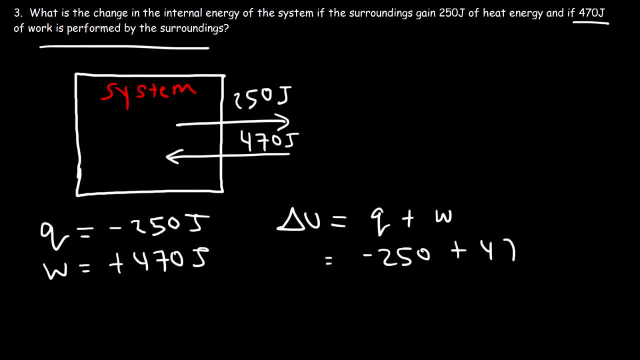 it's negative 250 plus 470.. So that's 220.. So I'm gonna clarify: If work is performed by the surroundings, the surroundings is losing energy due to work And that energy is going into the system, which means work is being done on a system. 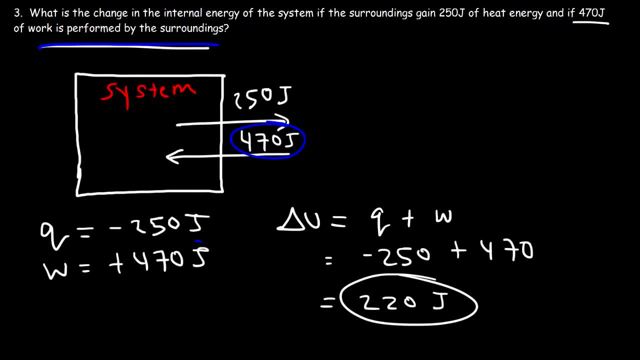 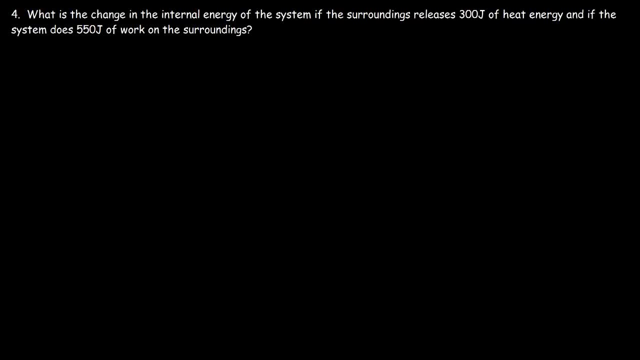 if it's done by the surroundings And anytime work is done on a system, W is positive. Number four: what is the change in the internal energy of the system if the surroundings releases 300 joules of heat energy and if the system does 550 joules of heat energy? 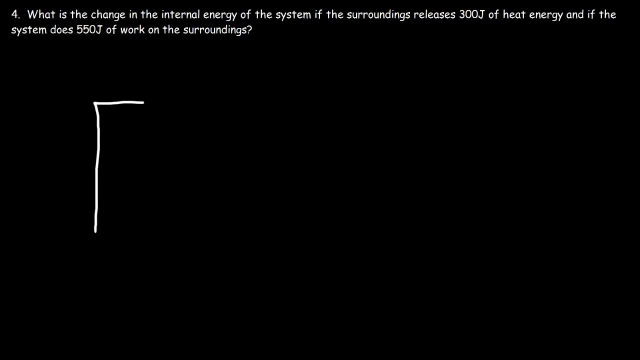 Well, if the system releases 300 joules of heat energy, the system is losing 150 joules of work on the surroundings. So go ahead and try this problem Now. if the surroundings releases 300 joules of heat energy, what does that mean? 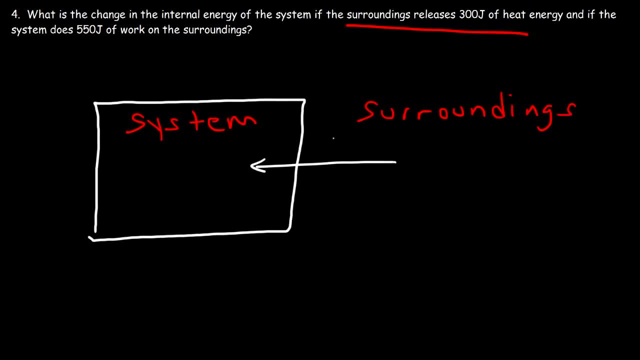 Well, that means the surroundings is losing energy, So the system is gaining that energy. So if the system absorbs 300 joules of heat energy, Q is positive 300. Now the system does 550 joules of work on the surroundings. 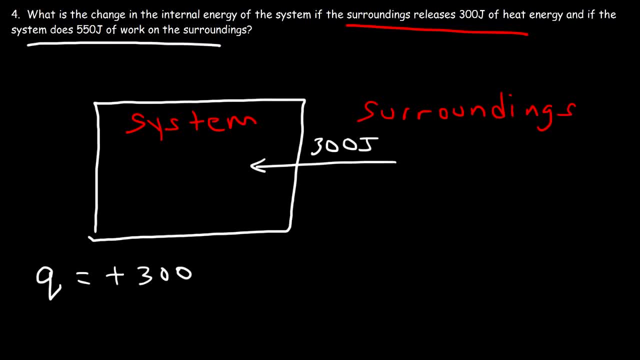 So work is being done by the system, but on the surroundings. Anytime work is done by the system, work is negative. Energy is flowing out of the system to the surroundings. So whenever work is done by something, energy is being consumed. 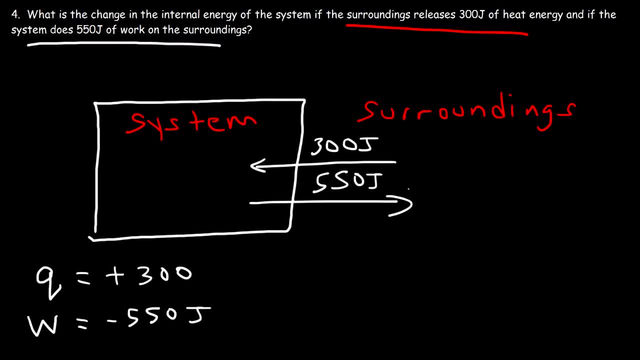 So if work is done by the system, the system loses energy. as it's doing work, It's expending energy, And if work is done on the surroundings, the surroundings is gaining energy. So make sure you understand what these expressions mean. So now let's calculate the change. 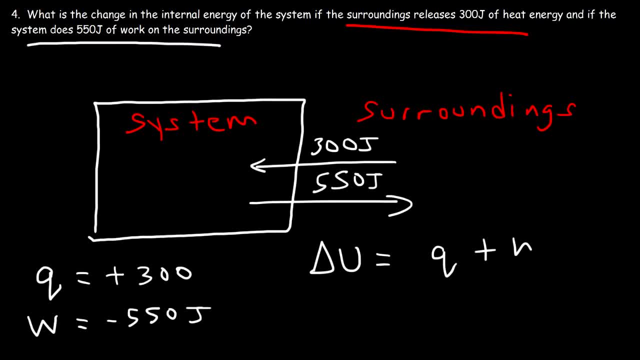 in the internal energy of the system. So it's Q plus W. So the system gains 300 joules. As you can see that's flowing into the system, But it's losing 550 joules. You can see that's flowing out of the system. 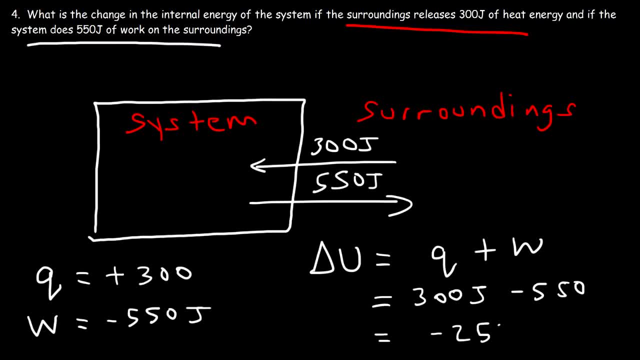 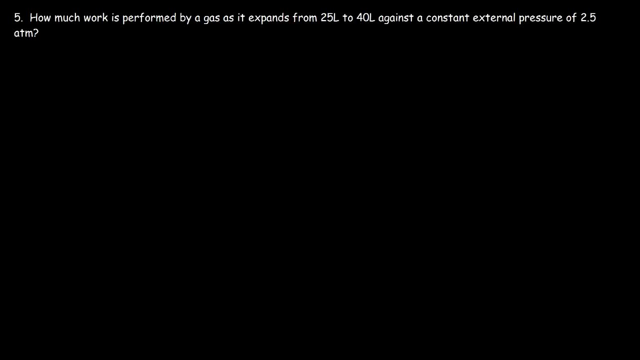 So the net result is that the system is losing 250 joules of energy. So delta U is negative. We got a net energy flow out of the system. Number five: How much work is performed by a gas as it expands from 25 liters to 40 liters? 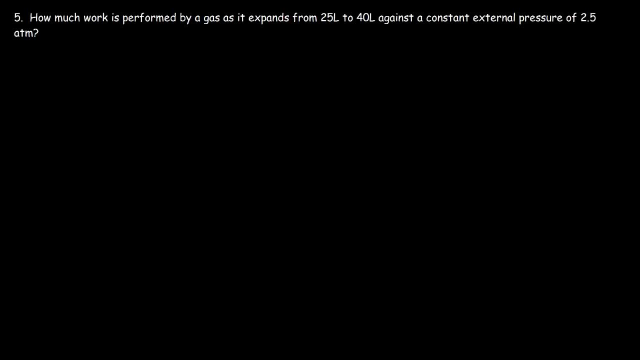 against a constant external pressure of 2.5 atm. So what equation should we use for a problem like this? Well, let's draw a picture. So this time the system is a gas. So let's say this cylinder is filled with gas particles. 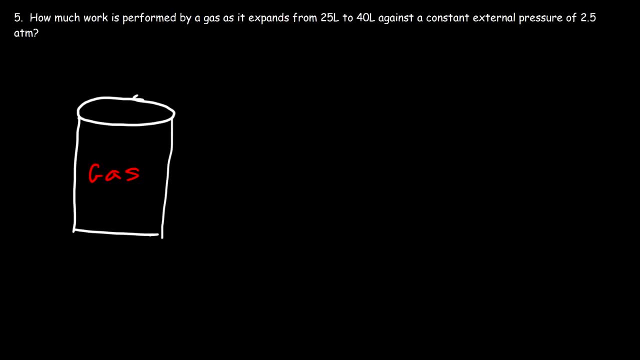 So that's the system, And outside we have the surroundings. Now the surroundings exerts a force on this gas. Any time you have a pressure, there's a force. Pressure is force divided by area, So there's a constant external pressure of 2.5 atm. 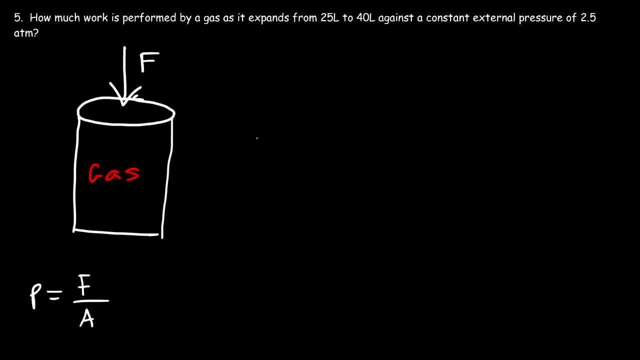 And that pressure exerts a force on the gas. As a result, the gas is going to compress And this problem is going to expand. but we'll talk about that later. Right now I'm just deriving the formula, So as we apply a force on a gas, 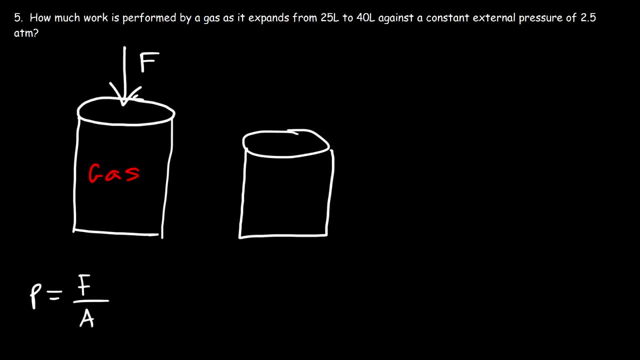 the gas will compress, So the volume is being reduced, And notice the change in the height of the cylinder. That's delta H. Now to calculate the work done, we're going to multiply the force by a gas or on a gas. 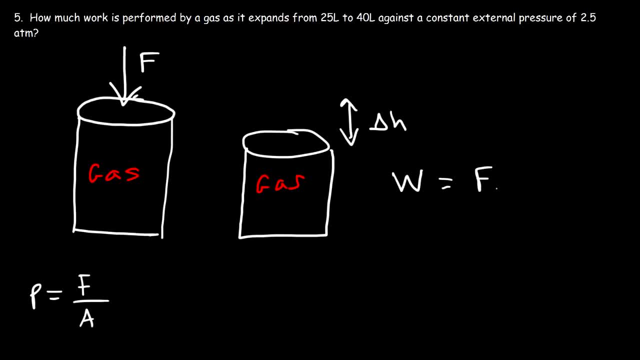 In this case it's on a gas, It's force times the displacement, which, in this case the displacement in the Y direction, is the change in height. And based on this equation, if you rearrange it, if you multiply both sides by A, 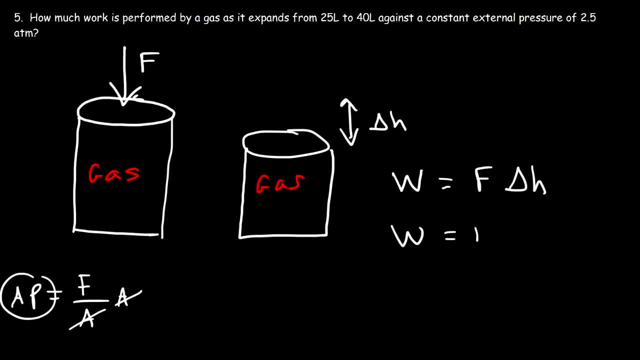 force is pressure times area. Now the volume of a cylinder is the area times the change or times the height. So area times height is the volume of the cylinder. The area is the area of this circle which is pi? r squared. So this is the volume of a cylinder. 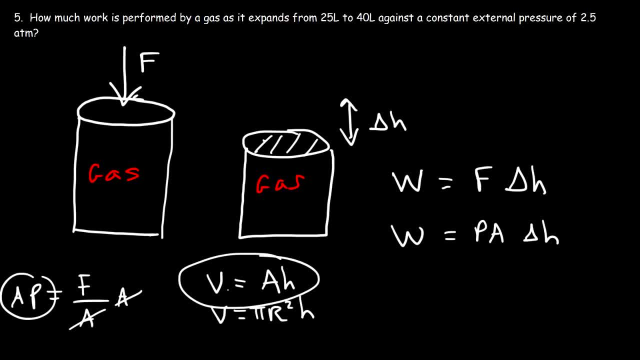 It's pi r squared times height. So if the volume is area times height, then area times the change in height must be the change in volume. Now we need to add a negative sign to make this work, Due to the sign conventions Now during compression, 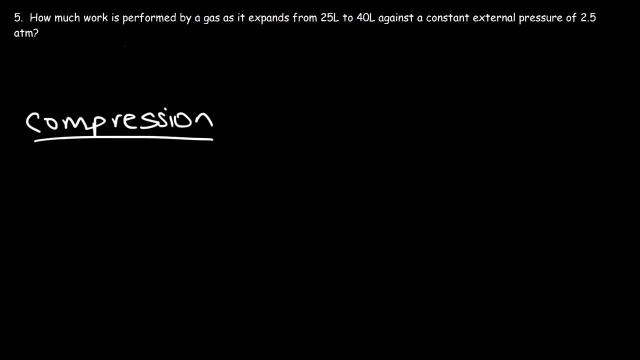 as was the case relating to the picture that we have. the change in volume is negative, The volume is decreasing And a force was being applied on the gas in order to compress it, So the surroundings was doing work on the gas, And whenever work is done on the gas, 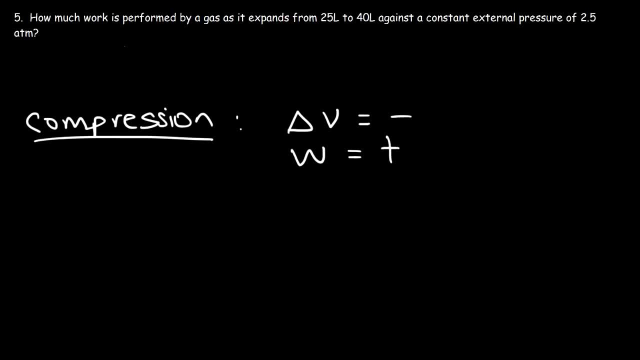 or on the system W is positive. During expansion, whenever a gas expands, the volume increases And the gas is doing work on the surroundings as it expands, And so work is going to be negative. So during compression, let me see if I can draw this picture here. 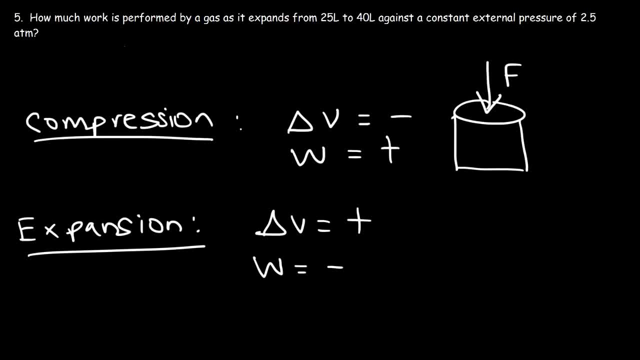 You're applying a force to compress a gas, So you're doing work on the gas, Which means you're increasing the internal energy of the gas. Whenever the volume decreases, the pressure increases, based on Boyle's Law. So as you apply a force to compress a gas, 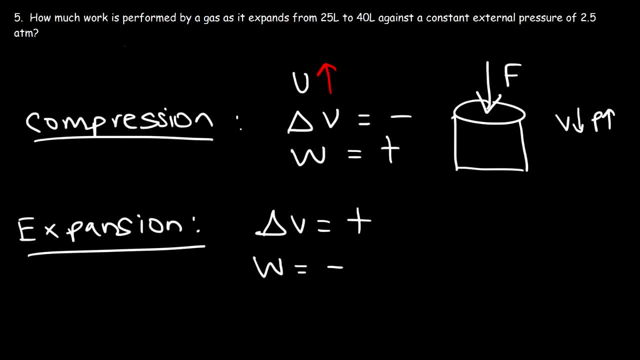 what you're really doing is you're expending energy, and that energy that you're expending, it's being stored in the form of pressure. So whenever you compress a gas, you're transferring energy to that gas, You're increasing its pressure. 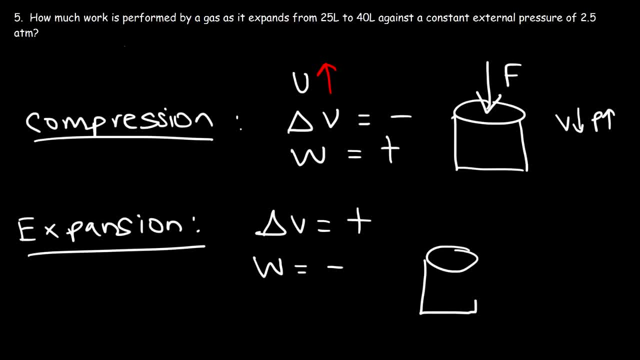 And whenever that gas decides to expand, it's going to apply an upward force, And as it applies an upward force, it can do work on the surroundings. So as the volume expands, the pressure reduces. So in order to store energy in a gas, 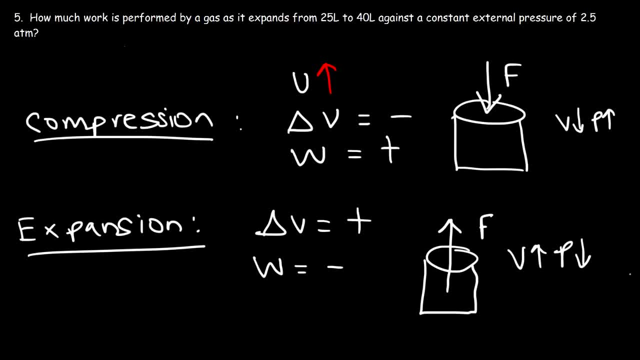 you need to compress the gas And to release that energy. the gas has to expand And keep in mind the energy is stored in the form of pressure, which is a type of potential energy. So gases that have a high pressure has a lot of stored energy. 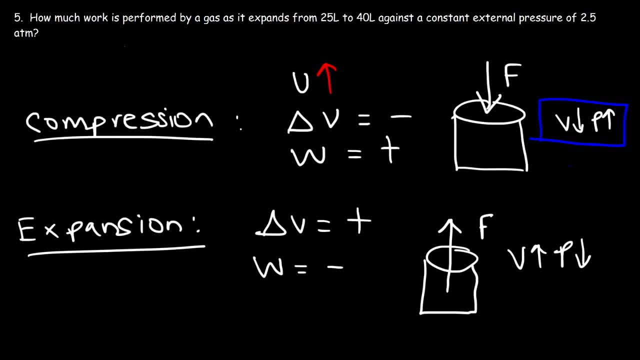 Gases at low pressure doesn't have much stored energy, So keep that in mind. So if you're doing work on a gas, you gotta apply a force, So energy is being transferred from you to the gas Now, as the gas expands against the surroundings. 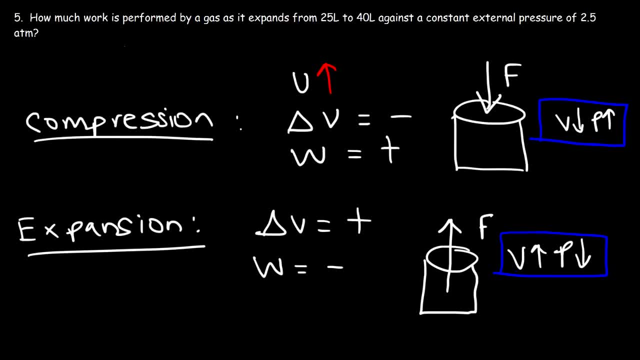 energy is flowing from the gas to the surroundings. So during compression, W is positive Work is done on the gas. During expansion, W is negative, Work is done by the gas, And so the internal energy decreases during expansion, but it increases. 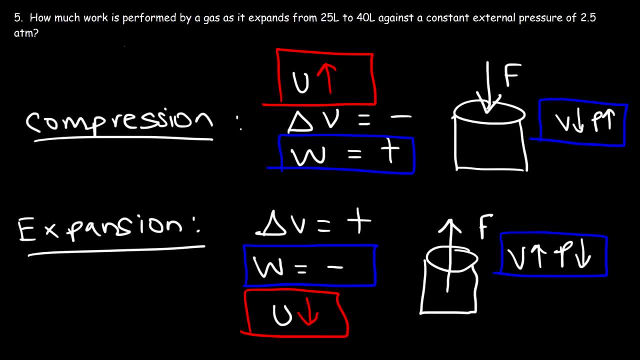 during compression. Now notice that delta V and W always have opposite signs. So, based on that, W is negative, P delta V. So when delta V is negative, you're gonna have two negative signs, which means W has to be positive, as in the case of this problem. 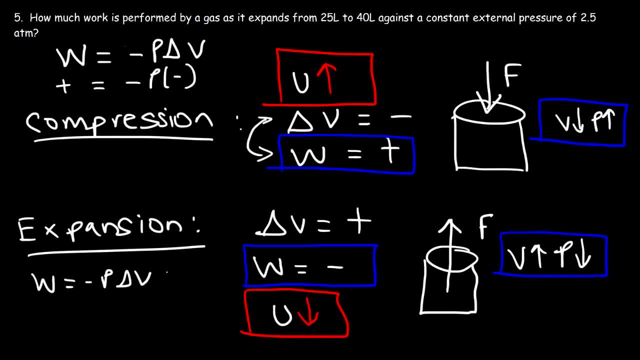 Or during expansion, when delta V is positive, W has to be negative, because a negative times a positive number equals a negative number, And so, because these two signs are opposite, that's why we have the negative sign in front of the equation. So just make sure you understand that. 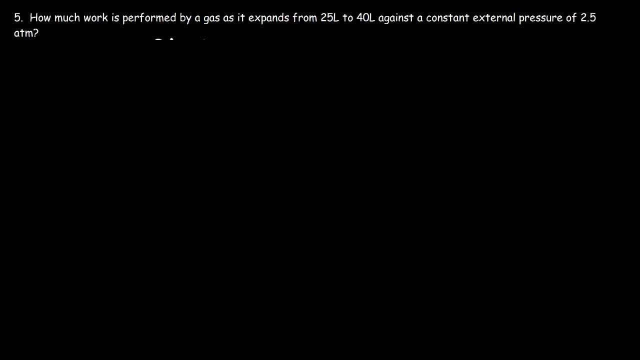 Now let's focus on a problem at hand: How much work is performed by a gas as it expands from 25 liters to 40 liters against a constant external pressure of 2.5 atm? So we said the equation is negative: P delta V. 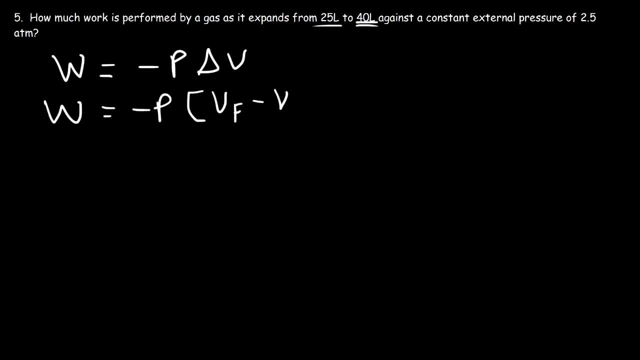 The change in volume is the final volume minus the initial volume. Now this pressure is not the internal pressure of the gas, because that gradually changes from 4 atm to 2.5 atm. P represents the constant external pressure that the gas has to work against. 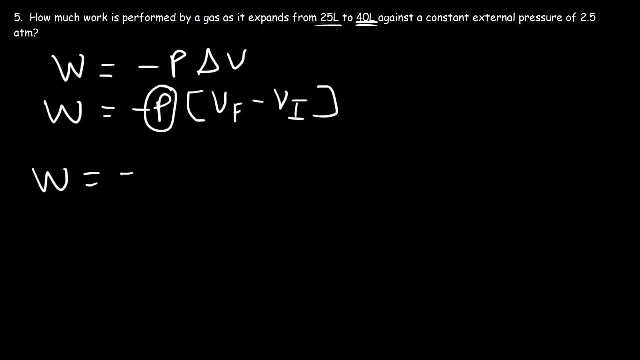 which was the 2.5 atm. The final volume is 40. The initial volume is 25.. So during expansion delta V is positive And we said W has to be negative whenever a gas expands. So 40 minus 15,. 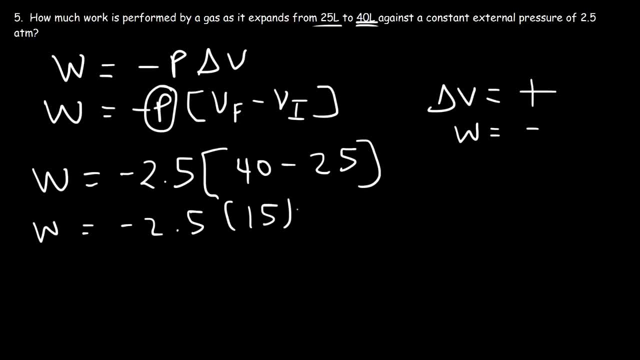 I mean 40 minus 25 is 15.. And 2.5 times 2.5 times 15, that's 37.5.. So the work is negative 37.5 liters times atm, Because the volume was in liters. 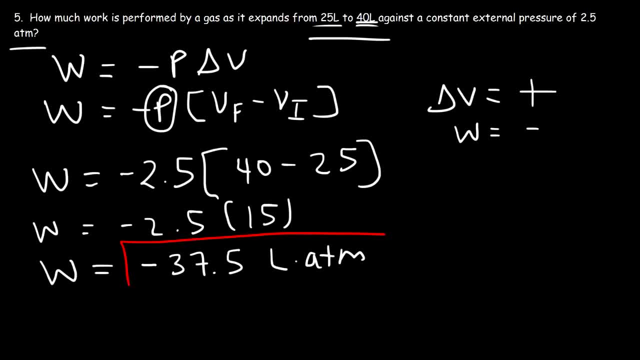 and the pressure was in atm. So anytime a gas expands, the work done by the gas is negative. Now you need to be able to convert this answer to joules, And here's the conversion that you need: 1 liter times 1 atm. 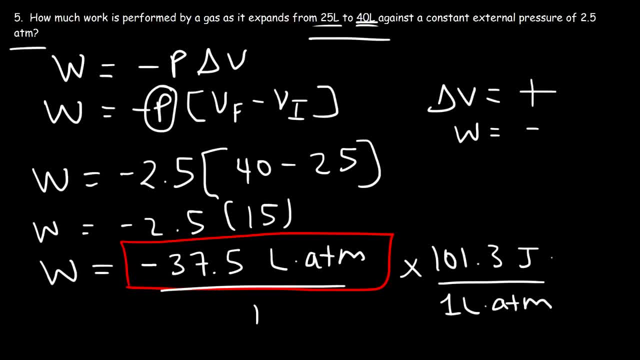 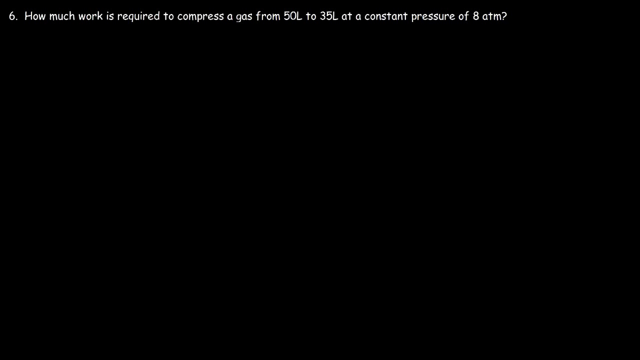 is equal to 101.3 joules, So W is 3,799 joules if you round it to the nearest whole number. And don't forget this is negative Number 6.. How much work is required to compress a gas from? 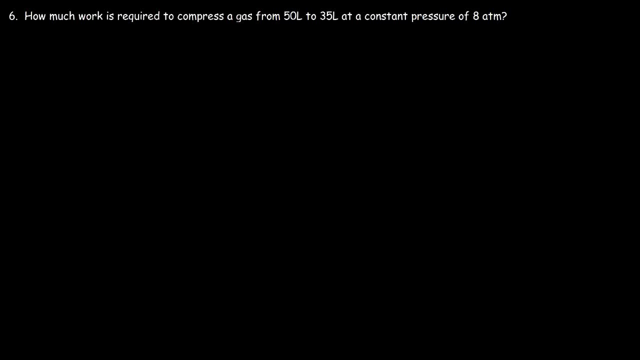 50 liters to 35 liters at a constant pressure of 8 atm. So during compression is the work going to be positive or is it going to be negative? To compress a gas, the work done on a gas is positive. The internal energy of the gas will increase. 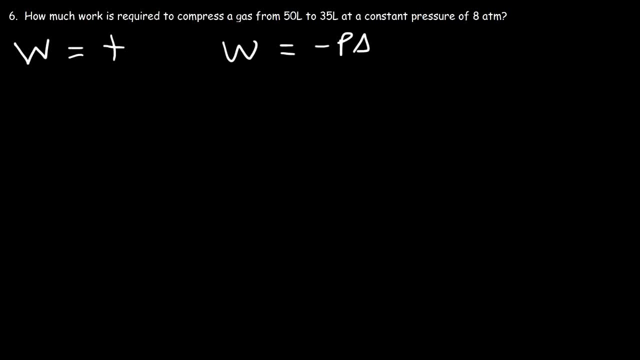 So let's go ahead and use this formula. It's negative P delta V, So the pressure is constant, It's 8 atm And delta V is the final volume, which is 35 liters minus the initial volume of 50 liters. So what we have is negative 8 atm. 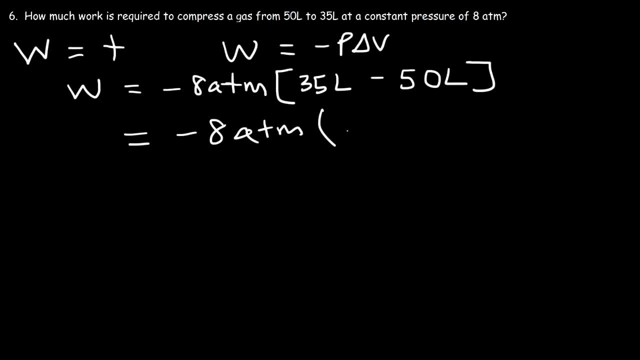 multiplied by a change in volume of negative 15 liters. So therefore the work required is positive 120 liters times atm. So now let's convert this to joules. So recall that 1 liter times 1 atm is equal to 101.3 joules. 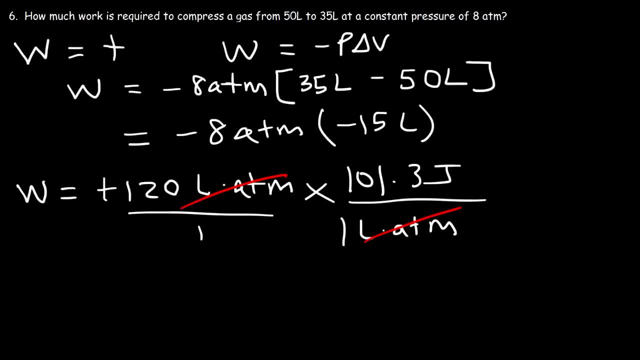 So these units cancel. So it's 120 times 101.3 and you should get 12,156 joules. So that's the work required to compress a gas from 50 liters to 35 liters at a constant pressure of 8 atm. 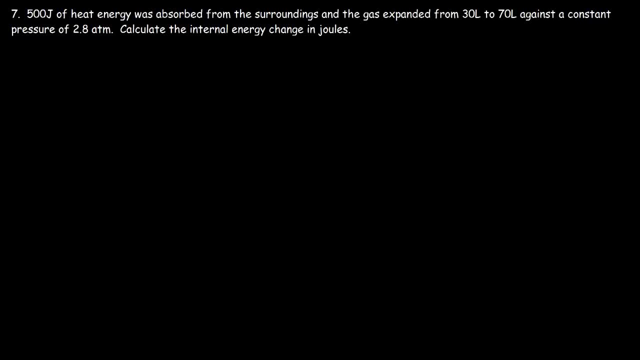 Number 7.. 500 joules of heat energy was absorbed from the surroundings and the gas expanded from 30 liters to 70 liters against the constant pressure of 2.8 atm. Calculate the internal energy change in joules. So let's start with. 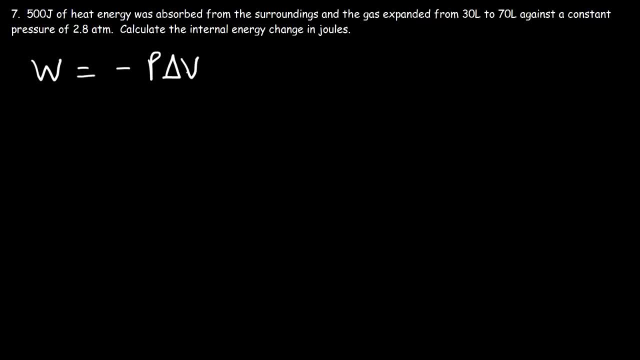 this equation, W is negative. P delta V, The change in volume is equal to the final volume minus the initial volume. Now the pressure is 2.8 atm And the volume, the final volume, is 70 liters minus the initial volume of 30 liters. 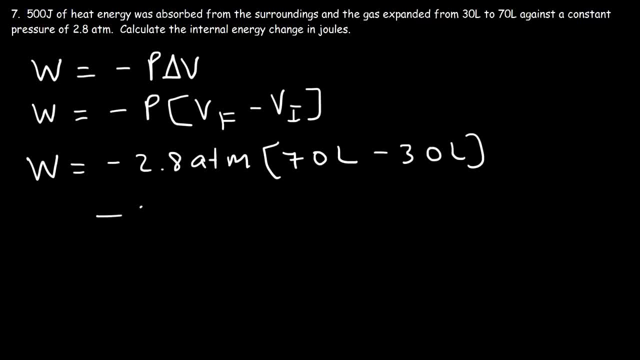 So 70 minus 30 is 40. So we have negative 2.8 atm multiplied by positive 40 liters. So the change in volume is positive due to the expansion of the gas, which means work has to be negative. So negative 2.8 times 40. 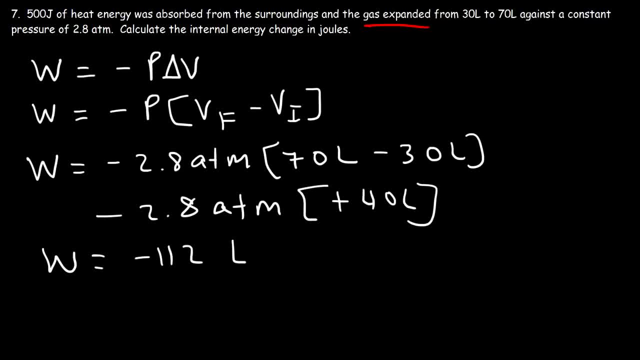 is negative, 112, with the units being liters times atm. And the last problem W was 120 and that was liters times atm. I didn't convert it to joules, but you know how to convert it to joules In this problem we need to.